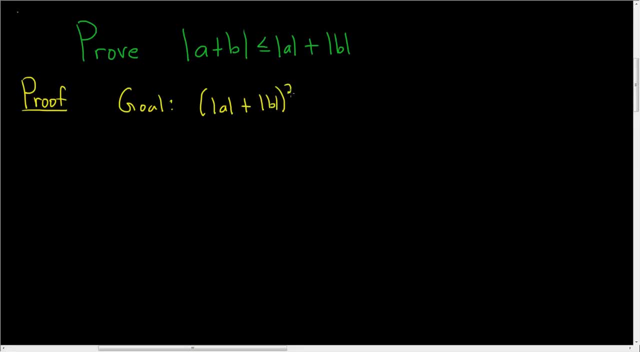 plus the absolute value of b squared is greater than or equal to the absolute value of a plus b squared. If we can prove this, then we can just take the square root of both sides and we get the above inequality and we're done. One useful fact that we're going to use in our proof is the following: Note that 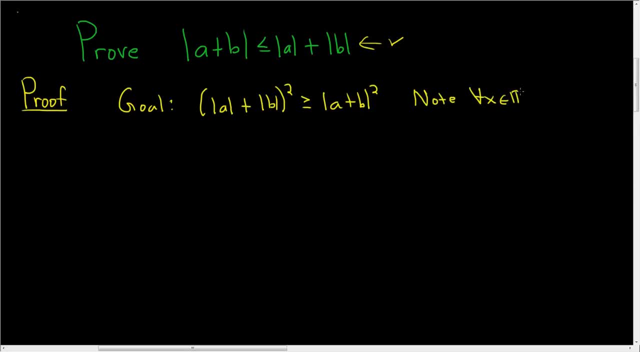 for every real number x. if you look at the absolute value of x squared, this is the same thing as x squared, So we're going to use this fact throughout the proof, So let's go ahead and do it. So for all real numbers a and b. 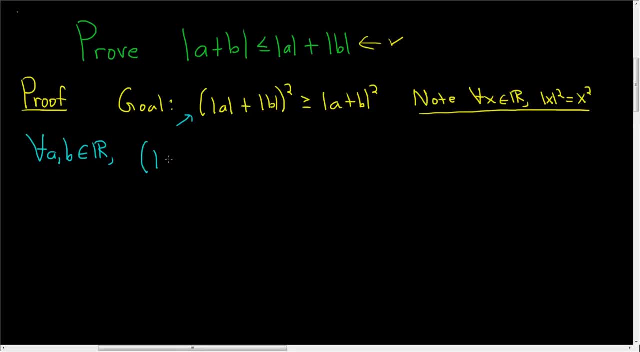 we're going to start by looking at this: Absolute value of a plus absolute value of b: quantity squared, This is equal to Well. there's a formula to multiply this out: You square the first term, you multiply these and you double it, so plus. 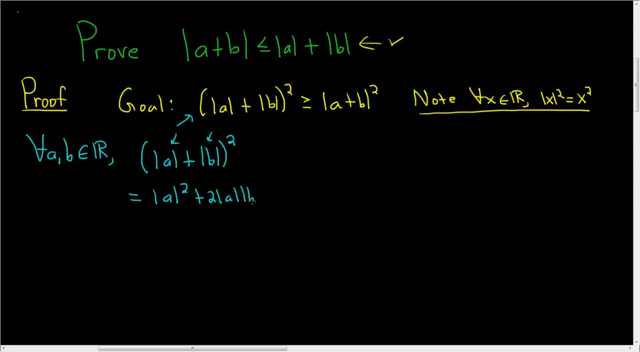 two: absolute value of a absolute value of b plus, and then you square the last term, So the absolute value of b squared, This is greater than or equal to. Well, we can replace the absolute value of a squared with a squared plus, And then we know that the absolute value of a is greater than or equal to a. 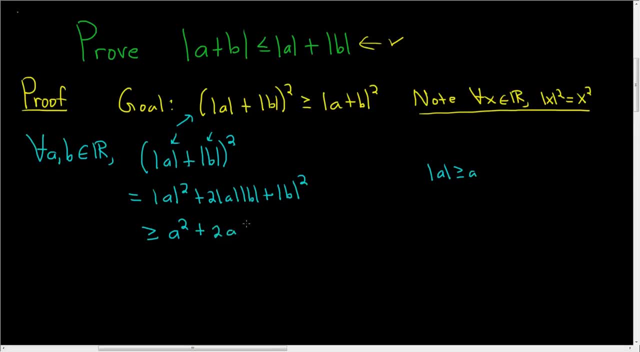 So we can replace the absolute value of a with a. Likewise, the absolute value of b is greater than or equal to b, So we can replace the absolute value of b with b. And again using this property, here we know that the absolute value of b squared is simply b squared. 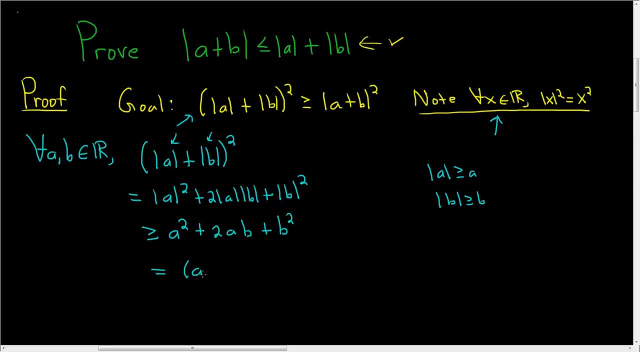 And so this is equal to a plus b, quantity squared. This is the same as the absolute value of a plus b squared. So we've shown that the absolute value of a plus the absolute value of b, the whole thing squared, is greater. 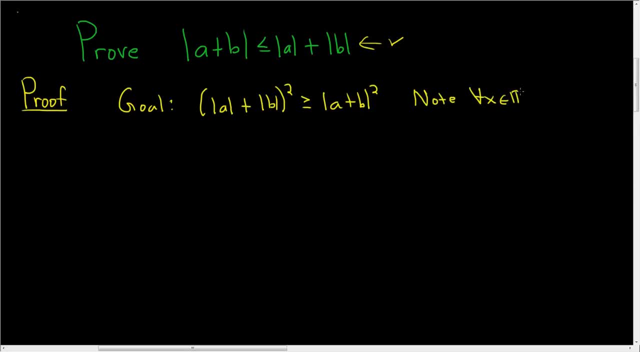 for every real number x. if you look at the absolute value of x squared, this is the same thing as x squared, So we're going to use this fact throughout the proof, So let's go ahead and do it. So for all real numbers a and b. 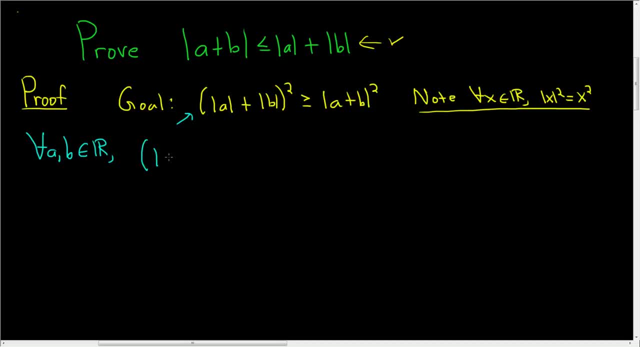 we're going to start by looking at this. so absolute value of a plus absolute value of b, quantity squared, This is equal to well. there's a formula to multiply this out: You square the first term, You multiply these and you double it. 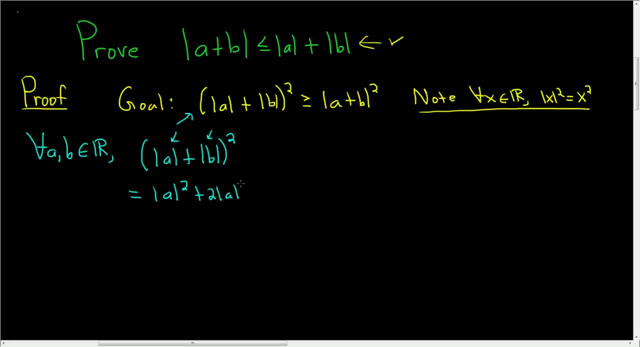 So plus two, absolute value of a absolute value of b plus, and then you square the last term, the absolute value of b squared. This is greater than or equal to, while we can replace the absolute value of a squared with a squared plus, and then we know that the absolute value of a is greater. 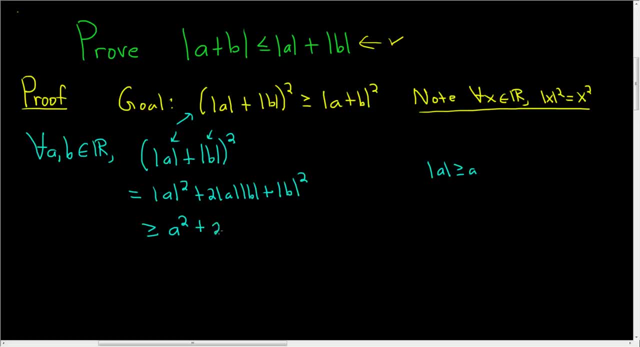 than or equal to a, So we can replace the absolute value of a with a. Likewise, the absolute value of b is greater than or equal to b, So we can replace the absolute value of b with b. And again using this property, here we know that the absolute value of b squared is simply b squared. 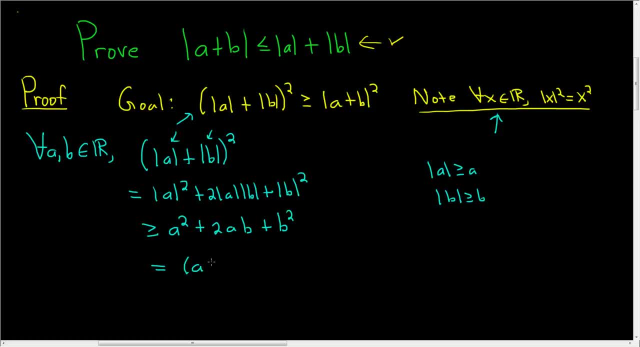 And so this is equal to a plus b quantity squared. This is the same as the absolute value of a plus b squared. So we've shown that the absolute value of a plus b squared is greater than or equal to b. The absolute value of a plus the absolute value of b, the whole thing squared, is greater than or. 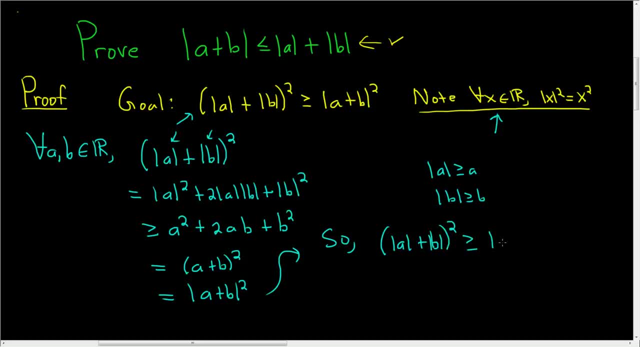 equal to the absolute value of a plus b squared. So now, if we take the square root, we end up with the absolute value of a plus the absolute value of b, greater than or equal to that- It est writing it backwards- the absolute value of a plus b. 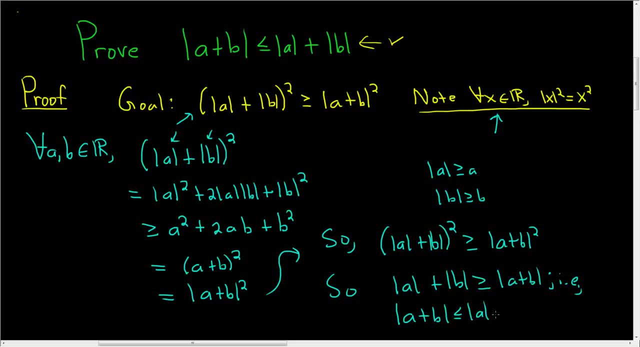 It is less than or equal to the absolute value of a plus the absolute value of b, And that completes the proof of what's called the triangle inequality. So this is probably the easiest way to prove it. I hope this video made sense. 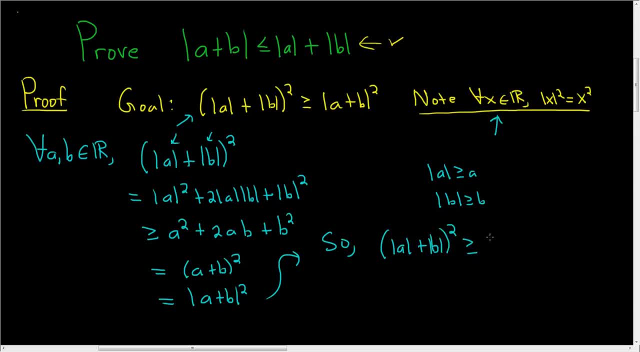 Greater than or equal to the absolute value of a plus b squared. So now, if we take the square root, we end up with the absolute value of a plus the absolute value of b, greater than or equal to that. It est writing it backwards: the absolute value of a plus b is less than or equal to the absolute value of a plus the absolute value of b. 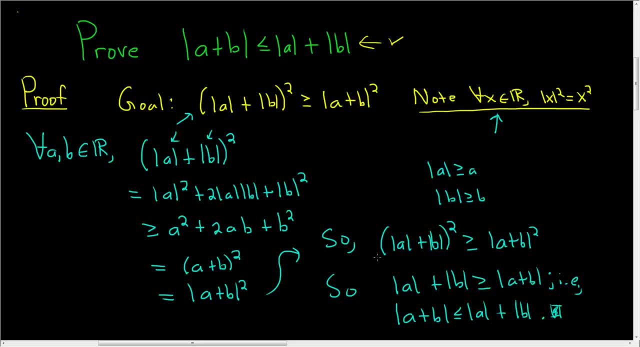 And that completes the proof of what's called the triangle inequality. So this is probably the easiest way to prove it. I hope this video made sense. 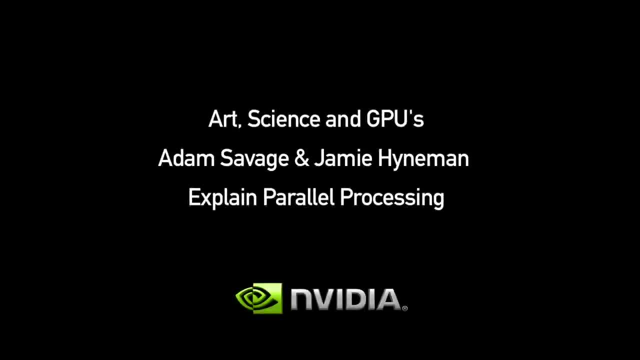 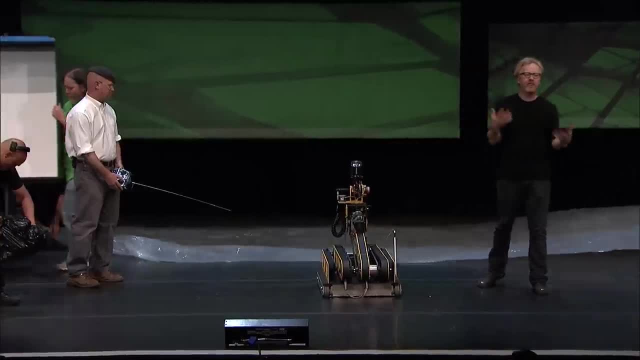 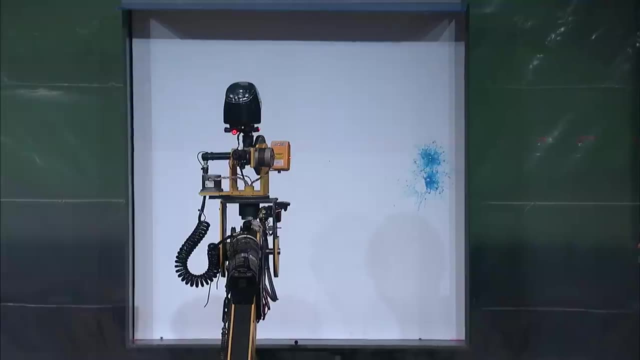 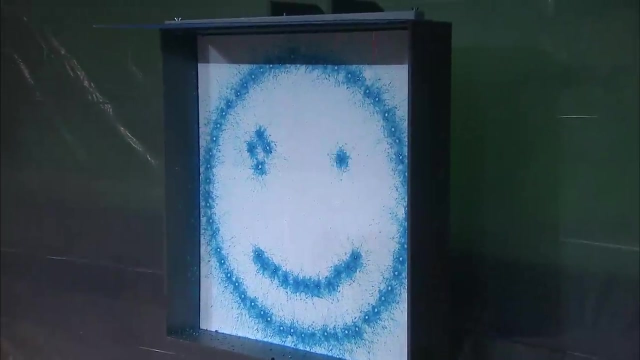 All right, I introduced to you Leonardo, and he's going to paint a picture for you guys, in the way that a CPU might do it, as a series of discrete actions performed sequentially, one after the other, In three, two, one. Let me speed it up. 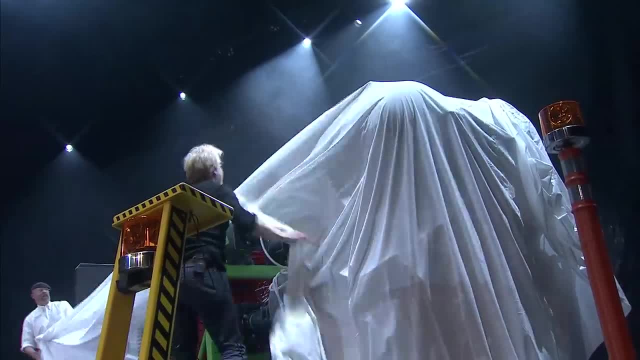 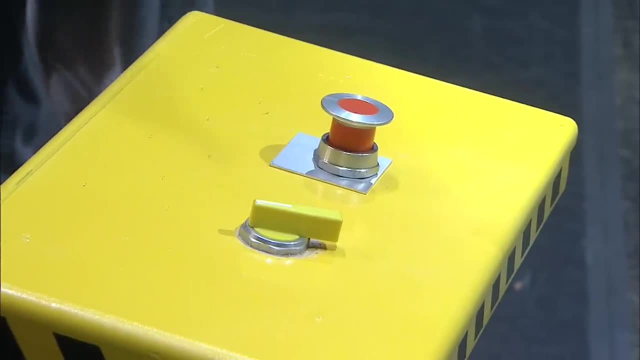 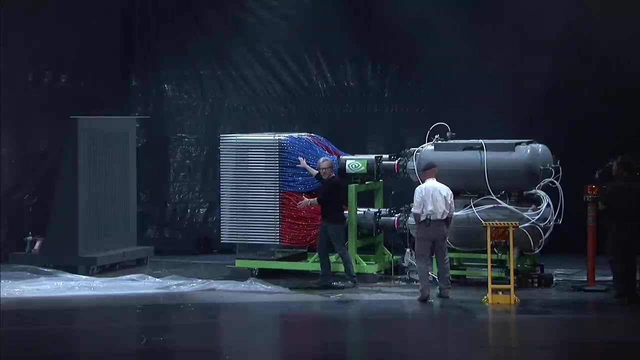 Ladies and gentlemen, Leonardo 10.0.. When we hit this trigger on this thing, 2,100 gallons of air goes through these accumulators, out these valves, into all 1,100 of these tubes, into these tubes in which the bottom of is a paintball, Each of those paintballs. 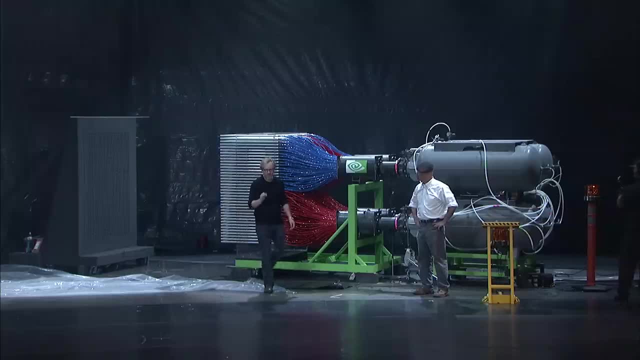 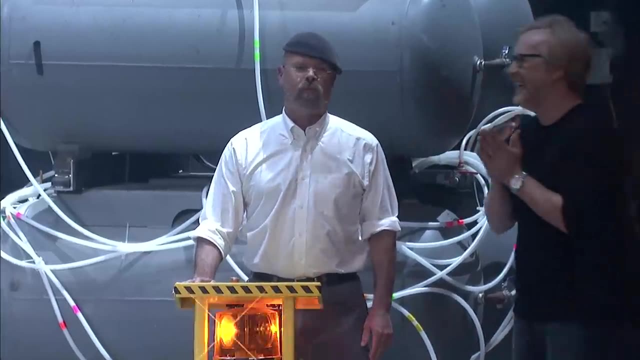 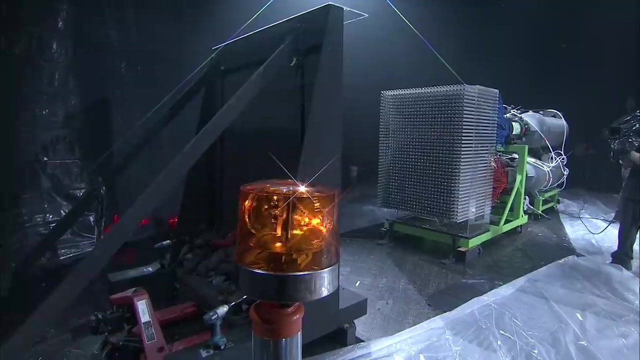 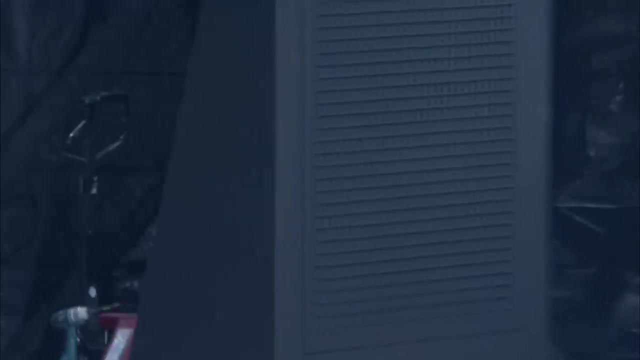 will fly across seven feet of space and, in 80 milliseconds, reach its target, hopefully, when it's all set. When it's all set and done, it's going to paint the Mona Lisa GPU painting demonstration in 10,, 9,, 8,, 7,, 6,, 5,, 4,, 3, 2, 1.. 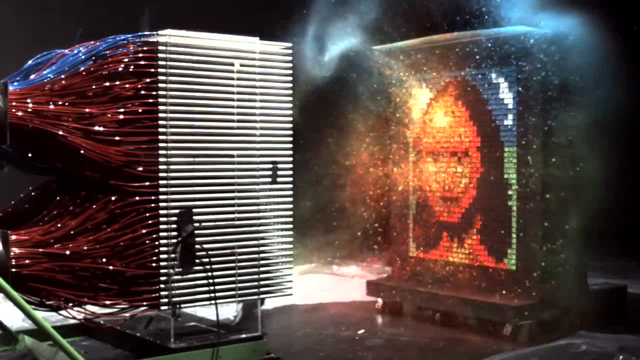 Ladies and gentlemen, science class is now over. Thank you, Thank you, Thank you.